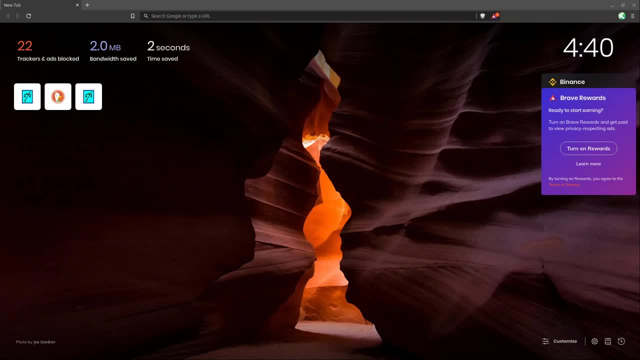 complex configurations is the Brave browser. However, it is worth noting that Brave has recently betrayed its users' trust in the past with what was essentially URL hijacking, by injecting their promo code into the URL of certain websites so that they could make a little bit more money. So it's important to keep a close eye on this Brave browser. 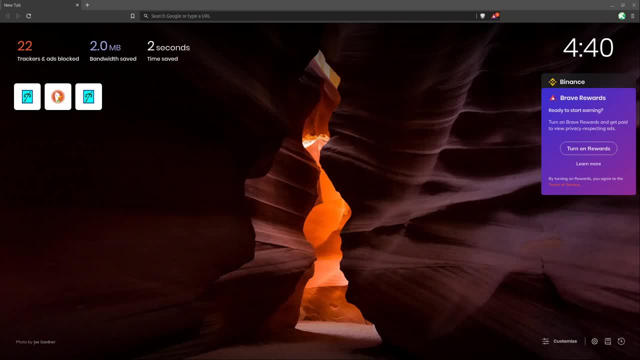 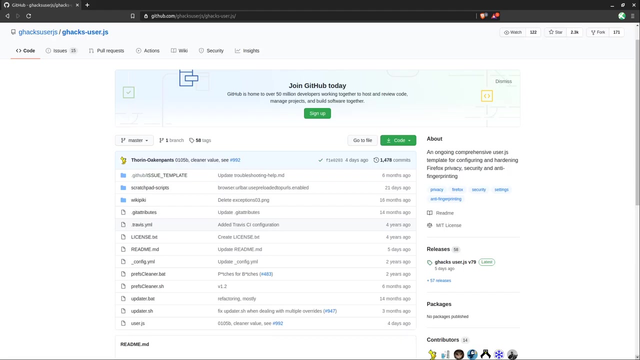 if you're going to use it and make sure that the developers never do anything like this again. But as of right now, I would say that it is the best browser that has good privacy settings right out of the box. If you're a more advanced user or you're just willing to do the extra work, that doesn't. 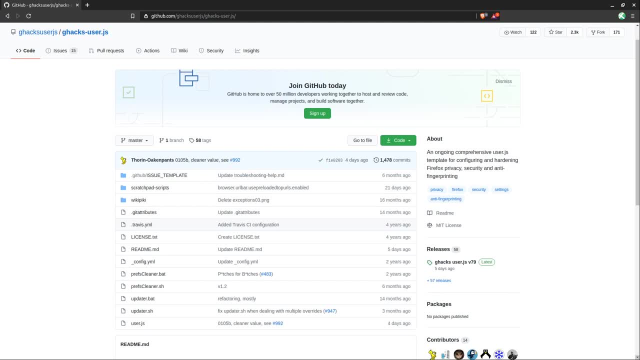 require trusting the Brave team, then you should use Firefox with the ghexuserjs profile to maximize the privacy of Firefox. You could also use ungoogled Chromium, which is an ongoing project to remove the spookiness from Chromium and allow its users to browse with. 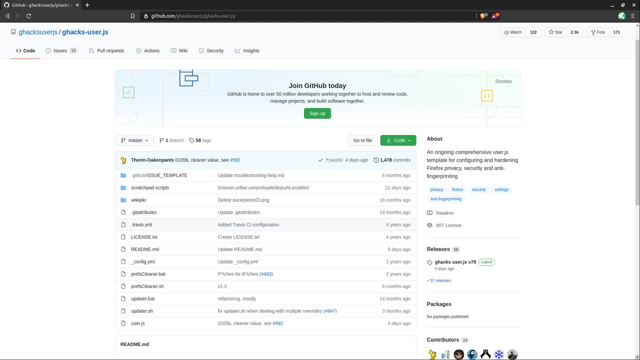 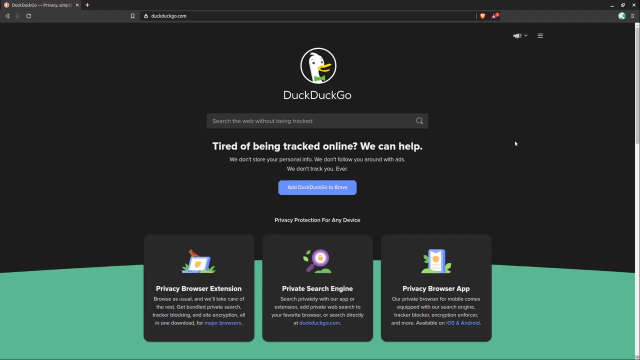 without Google spying on them. However, you should still install a couple of other add-ons to ungoogle Chromium, like uBlock Origin. Now, when you're on the web, you probably use a search engine quite often, So it's important to use a search engine that respects your privacy. The one that I would recommend is: 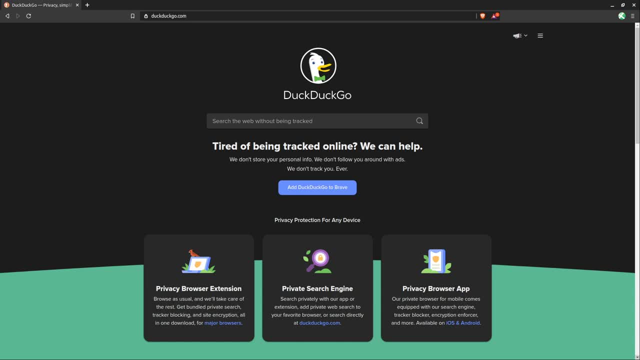 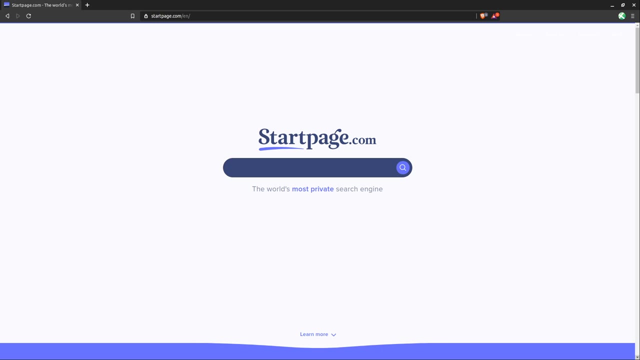 DuckDuckGo. They have a long track record of respecting a user's privacy. However, DuckDuckGo occasionally has insufficient search results, depending on what it is that you're looking for. So if you find this to be an issue, you could use StartPage, which generates results from 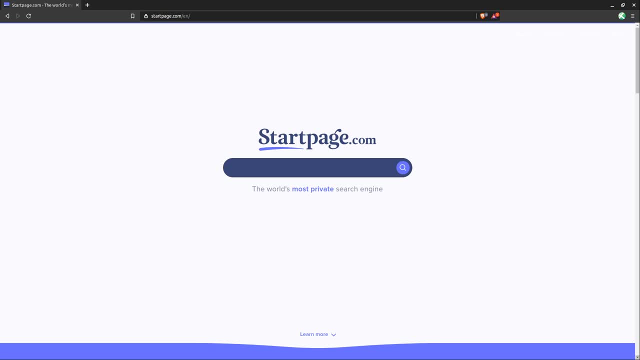 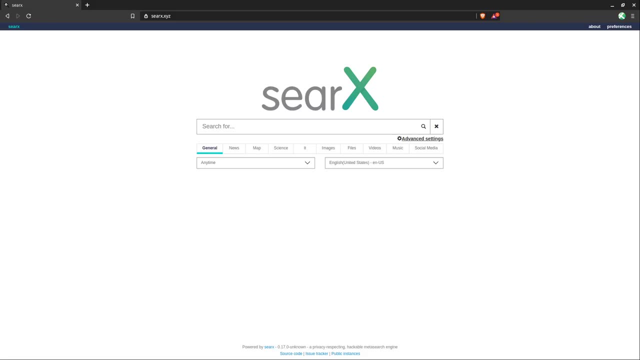 Google, while having more respect for the user's privacy than using Google directly. Or if you want to take things a step further, you could use Surex, which gives you the option to use a vast number of privately hosted instances or to host your own instances. 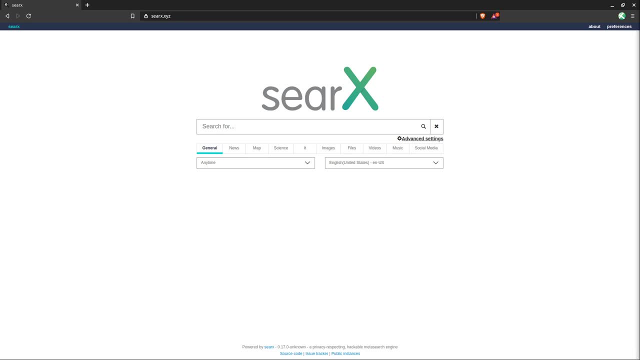 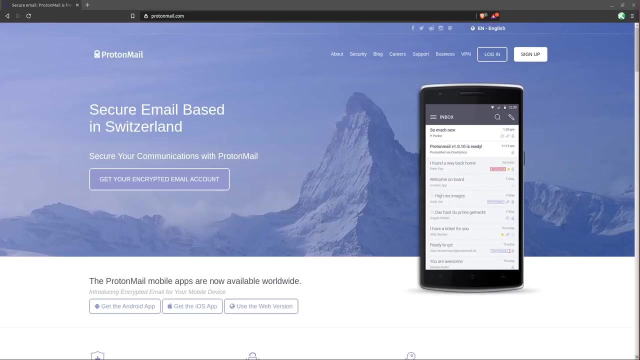 Also, this is probably the best way to achieve a balance of privacy and to avoid search results being manipulated, which Google, Yahoo and other big search engines are well known for doing. Another activity that many people use their web browsers for is email, Even if you don't. 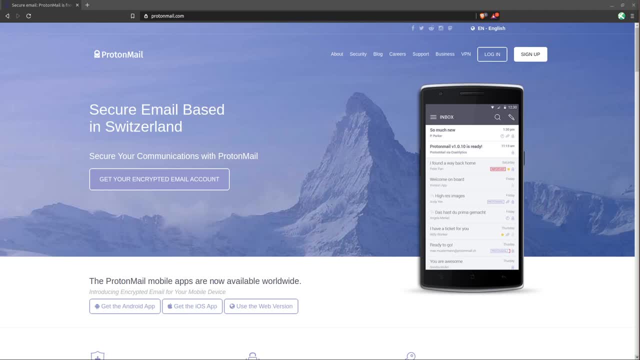 enjoy using email. it's still a necessary evil because most services still require either a phone number, two sign-ups or a password. So just use your phone number and you're good to go, or an email to sign up for them, And obviously emails can be much more anonymous than a phone. 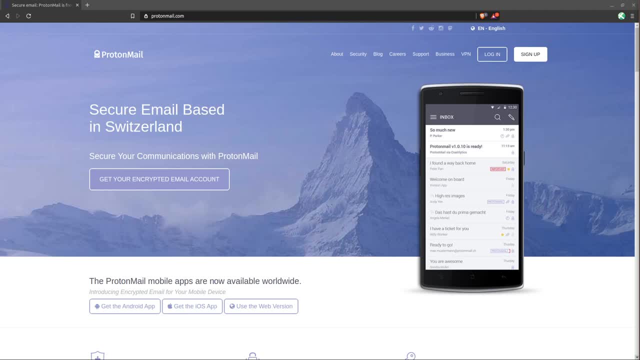 number, But if you're going to use email, it's important to use an email provider that respects your privacy. This means that Yahoo Mail, Gmail and Hotmail are all out, because all of these services make a profit off of selling your data to advertising companies. You should use an email. 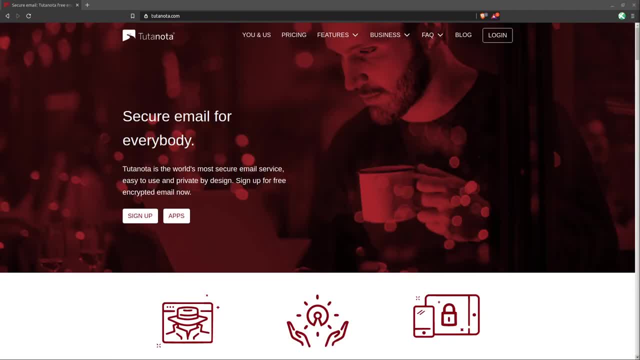 service like ProtonMail or Tutanota, which has been proven to have a track record of respecting user privacy, And they are both able to do this because they encrypt your inbox. So even if these companies wanted to monetize your emails and make profit off of your inbox, they wouldn't be able to. 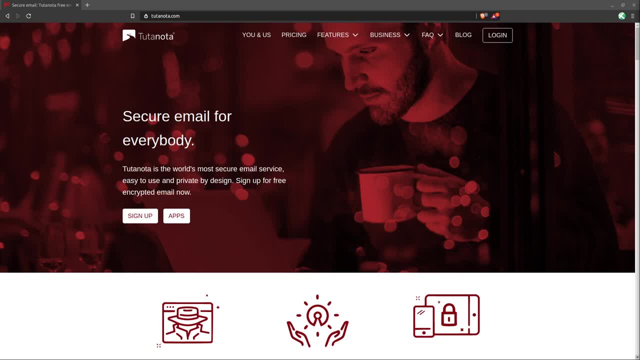 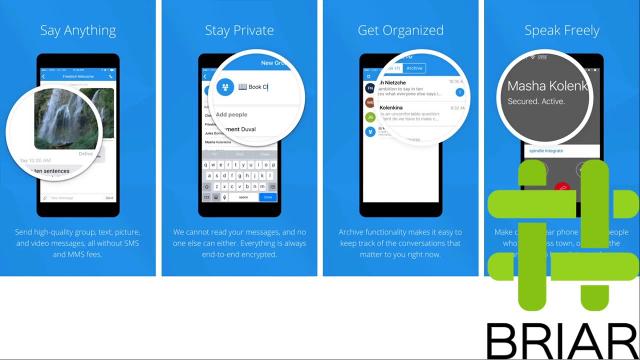 do so because the contents of your inbox are hidden from them And they're only viewable by you when you sign in with your password, which decrypts them. You should also use a secure and privacy-respecting means of communication for all of the other ways. 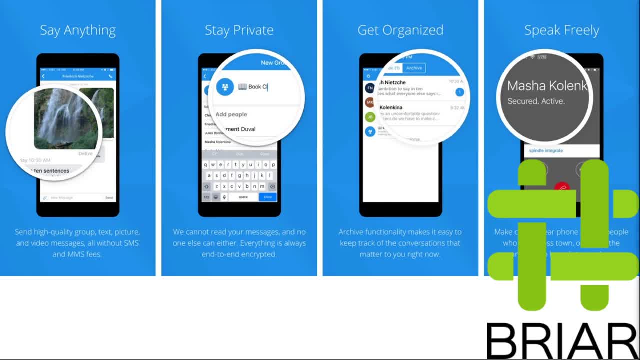 that you want to message people. So for instant messaging, I would recommend using either Signal or Briar. Both of these support end-to-end encryption. They are both free and open source, And Briar goes a step further by sending messages through the Tor network to further obfuscate the communication between the two companies. So if you're going to use an email service, you should also use a secure and privacy-respecting means of communication. Both of these support end-to-end encryption. You should also use a secure and privacy-respecting means of communication between the two companies. 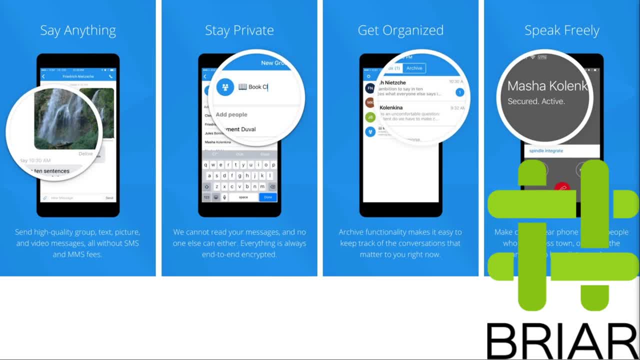 You should also use a secure and privacy-respecting means of communication between the two companies, And neither of these companies store your data or your metadata, And even if law enforcement were to subpoena them, the most that they could give up is the date that you created your account and when. 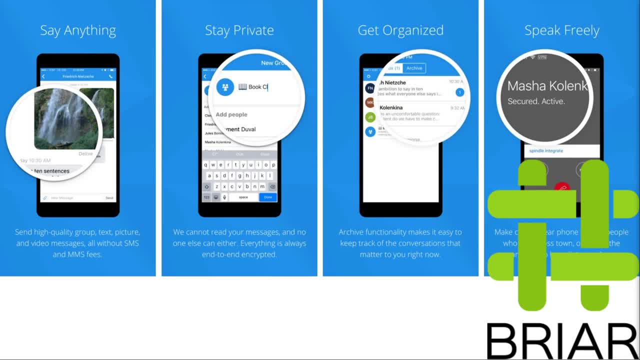 you last logged in, since they don't keep any logs of your usage history And both of them support end-to-end encryption, So there's no way for them to actually see the messages that you were sending back and forth. And both of these apps are very easy to use. So if you're going to use a secure and 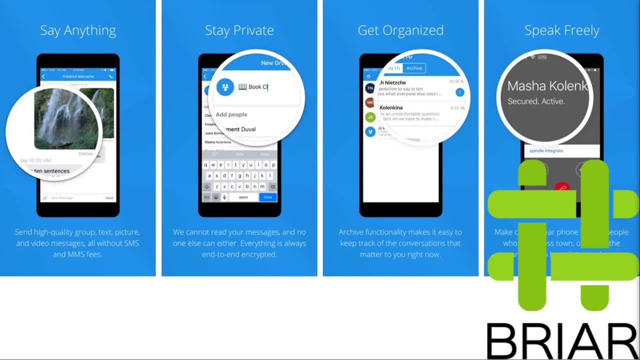 both of these apps are available on a wide array of mobile and desktop platforms. the only real struggle here is getting your friends to use them as well, since obviously both parties must be using this app in order to benefit from all of this privacy. Now, when it comes to digital and online security and privacy, there are many layers involved, And 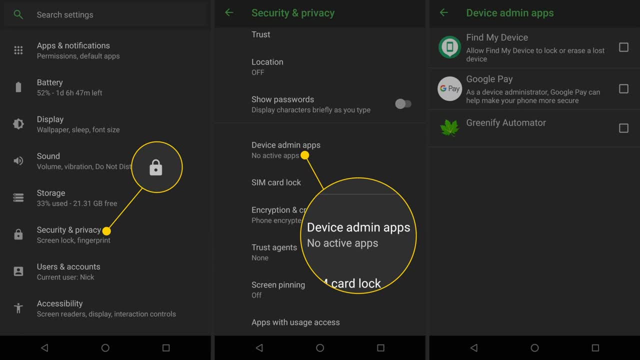 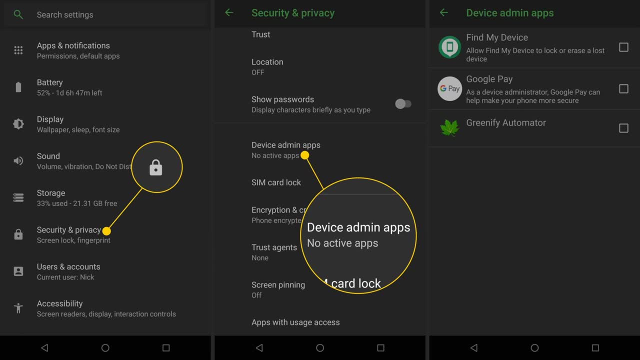 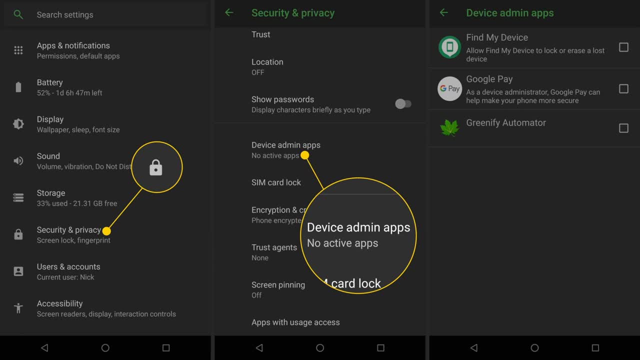 secure by default. it is important to then go and secure the settings of your operating system. The default settings of most operating systems, especially mobile ones, are not privacy-oriented. So on your desktop or your mobile platform, you should disable things like data sharing, location services, error reporting, usage statistics, anything. 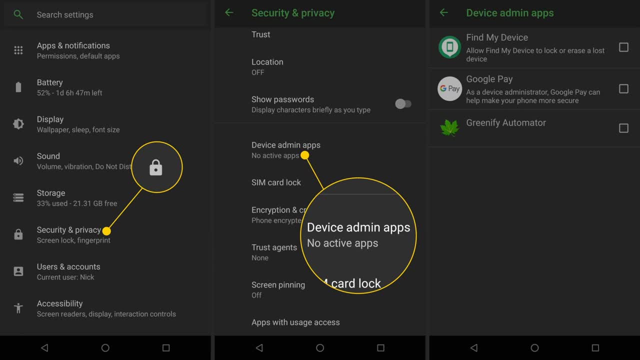 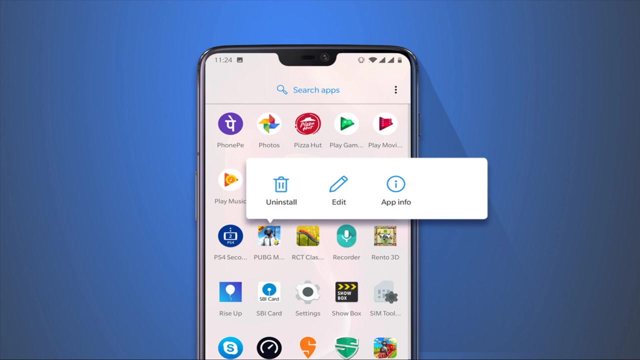 like that that sends data back to the proprietor or to an advertising company, should be turned off within your operating system and your online services. And, speaking of online services, you really should limit the number that you're using, as well as the number of apps that you're using. 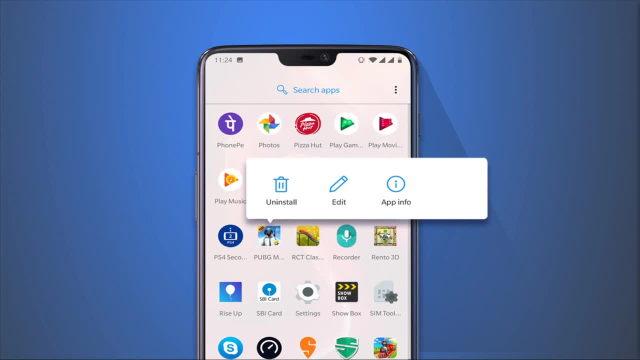 or that you have installed on your device, because chances are you have a number of apps on your phone that you don't even use, but they are still going to be collecting your data in the background. when you give information to multiple applications, This goes and enlarges your digital footprint, and 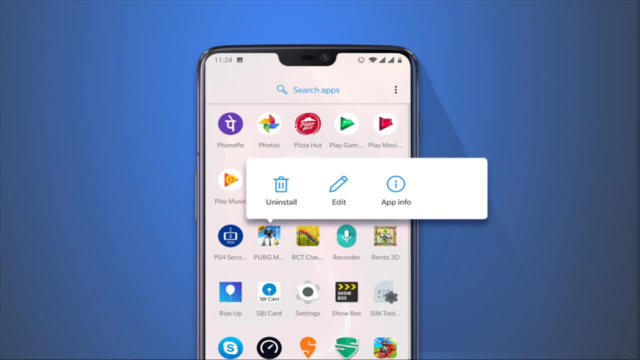 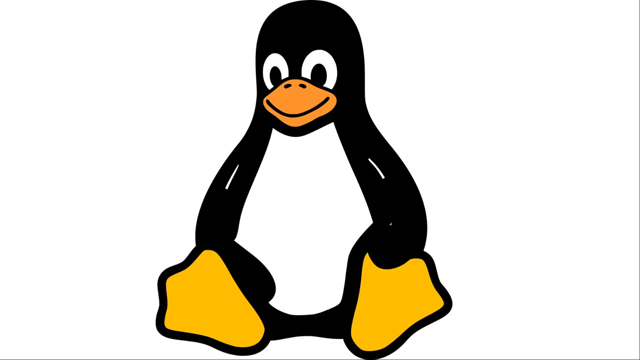 it's giving out more information to anybody that can access this data, either through hacking or through buying it from the proprietor of these apps or the proprietor that makes these apps themselves. And number seven: you should run your browser, your browsers, your apps and your online services from a free and open source operating system. that 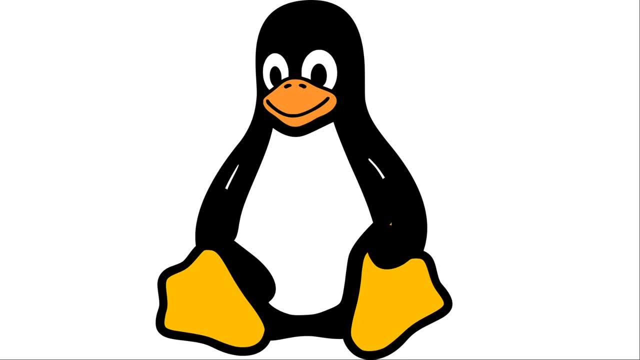 respects your privacy. As I mentioned earlier, if the layers below are unsecure, then the layers above are going to be compromised and generally the operating system is the lowest level software that a user would interact with. If you run a close source proprietary operating system like